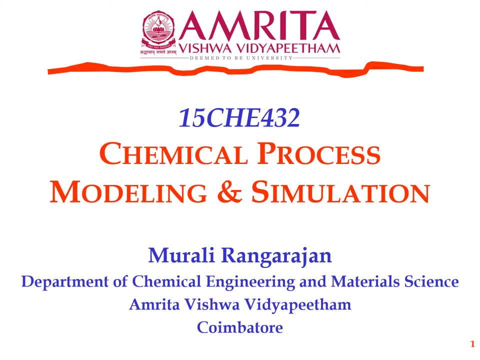 introduction to what modeling is all about, what are the different types of models, how modeling plays a role in daily life. We looked at different examples through which we understood that In this lecture we are going to see what is mathematical modeling and what are the different types of. 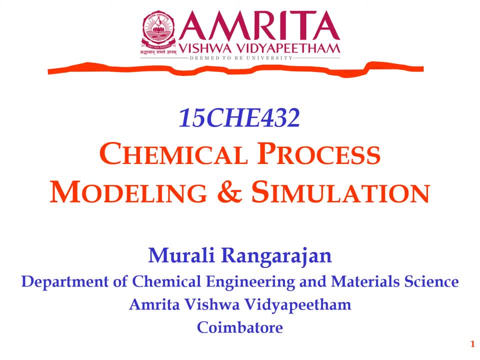 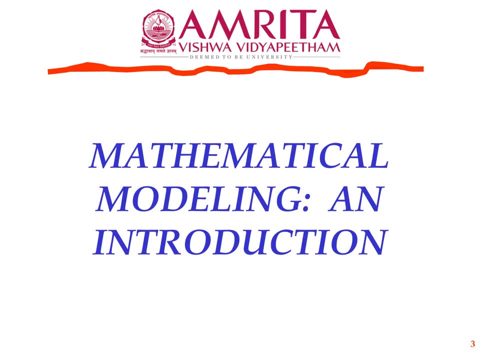 mathematical models and what are the different types of mathematical models and what are the different methods applied, and we will see a practical example of mathematical model. So the lecture I am going to start with a mathematical model that I put up in the previous lecture, which is the mathematical model of a crude distillation unit. 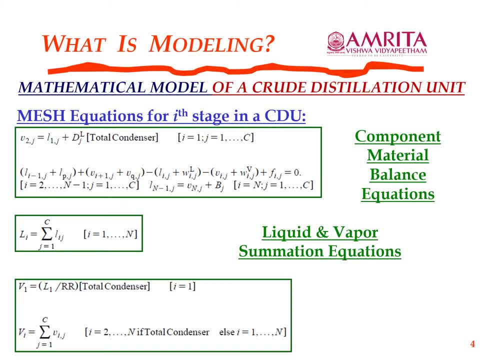 This is the model equations for a crude distillation unit at the city Distillation unit at The, The, The Indian Oil Corporation's Mathura Refinery in India, Mathura in India, and we have the component material balance equations, liquid and vapor, summation equations, enthalpy or 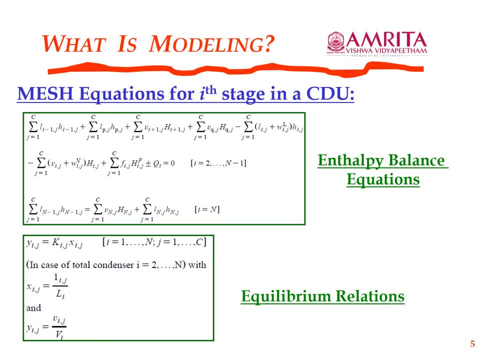 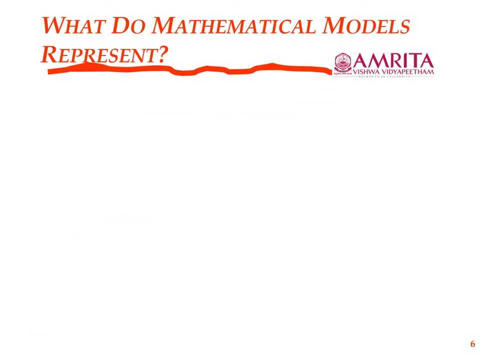 energy balance equations and equilibrium relations. This is for any ith stage of the CDU, or the crude distillation unit J denotes the subscript, J denotes the various components. so there are N stages- I going from 1 to N, and C components, J going from 1 to C. Well, so we saw a mathematical model like this: 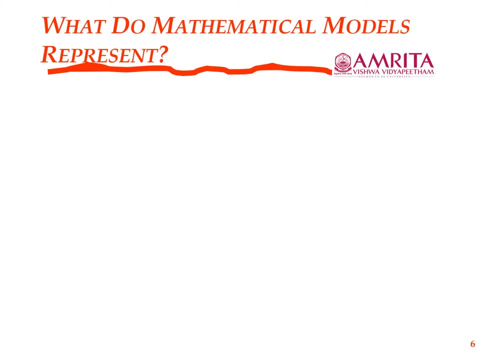 So what do these mathematical models represent? Mathematical models are approximate mathematical representations of processes Occurring in a unit or a set of units. So if you are writing a mathematical model for a single unit, like, for example, the atmospheric crude distillation unit, So this set of equations that we saw there represent, of course mathematically, because 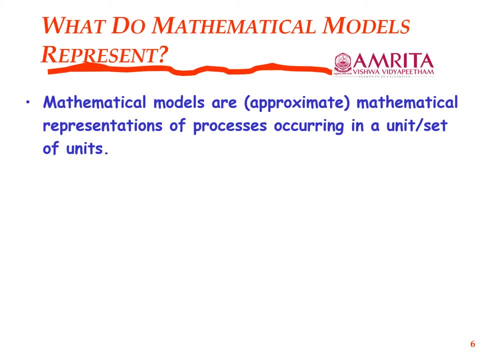 these are equations, the processes that are occurring in that atmospheric crude distillation unit. What is the process, Basic process that occurs in the Okay, In the CDU? it is one of distillation where the low volatile component is volatilized and 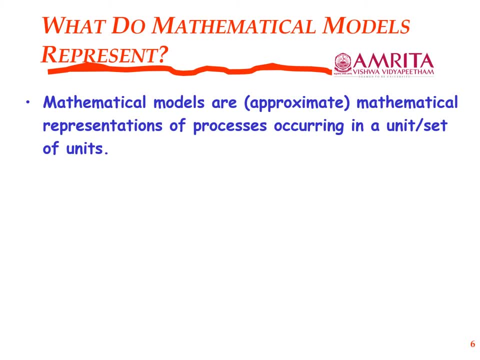 moves upward, from bottom of the unit to the top of the unit, and that is predominantly in the vapor phase, and the heavy components, which are predominantly in the liquid phase, flow down. the heavy volatile components, the less volatile components, rather than the liquid components, rather than the heavy components. they condense from the vapor phase and they 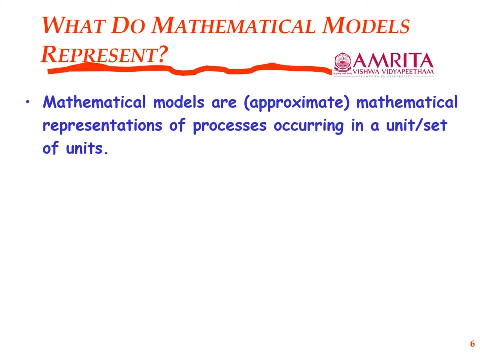 get collected, accumulated in the liquid phase and they keep coming down. and, as with any crude distillation unit, there are multiple products. So at different intermediate stages there are products that are, that are moved, and then there are additionally side strippers when the products liquid stream is removed there. 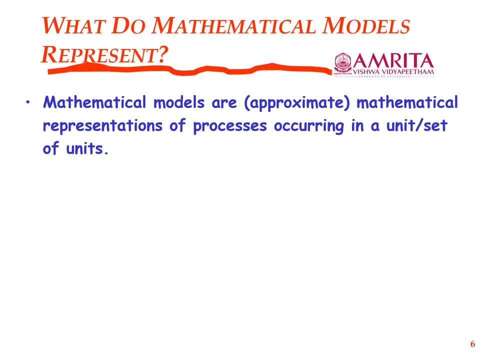 is a mini, small distillation column in itself Where there is this, you know, further enrichment of the product, that is, that is basically to be collected from that stream and then the remaining part of it is sent back to the column. So there are multiple side strippers and there are what are called pump arounds to ensure 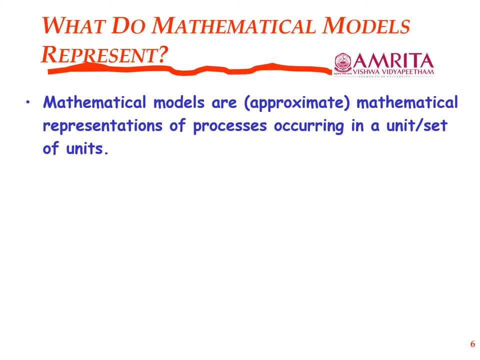 basically, some liquid is taken from a lower stage and then pumped back up to a higher stage Which, even though You know, It sort of overrides any separation that has achieved. that has been achieved by the liquid coming down. it is now being put back up right and that separation is lost. however, it ensures 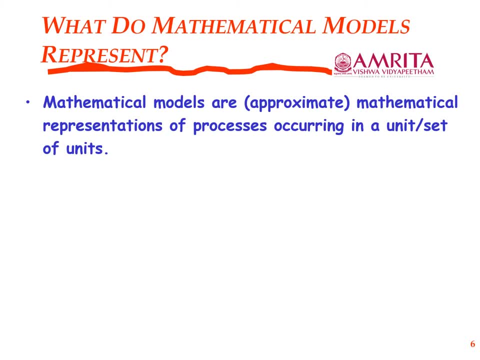 that there is sufficient amount of liquid in all the stages, and also it sort of in in distillation processes such as that of crudes. you know, since no product is a pure component, they are all cuts. So it ensures that there is sufficient amount of liquid in all the stages. 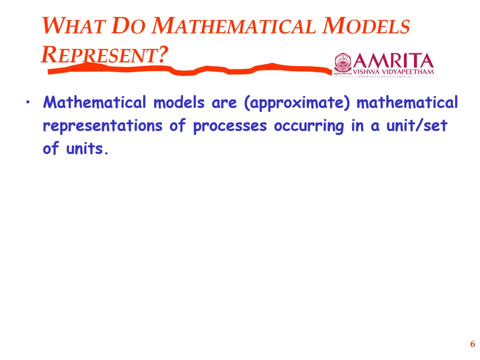 So it ensures that there is sufficient amount of liquid in all the stages. So it ensures that there is sufficient amount of liquid in all the stages. So it ensures that there is sufficient amount of the distribution of the various components that are present in a cut by its pump arounds. 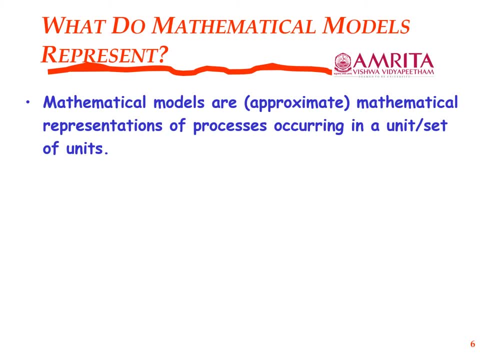 So all these are there and the equations were written that that essentially captured All these processes. So, essentially, the flow of the vapor up the column, flow of the liquid down the column, the equimolar or non equimolar counter diffusion that takes place between the vapor and the 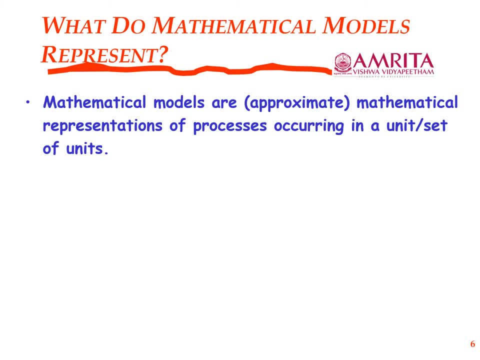 column liquid phases in each stage and and then there may be some sort of a stream coming in due to a pump around, or going out, or coming in due to a side stripper, and the various product streams that are excited at different stages. that is, a feed that comes in at a feed stage. all this are all. 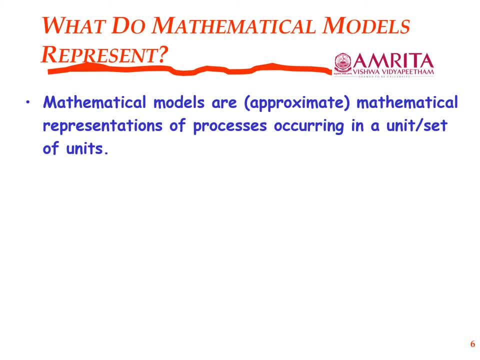 processes that take place, number one and number two. in addition, this mass transfer process occurs, goes to a point where you know the, the hope, the, the idea, that stage is designed to reach as close to an equilibrium between the vapor and liquid phases as possible, and this equilibrium is: 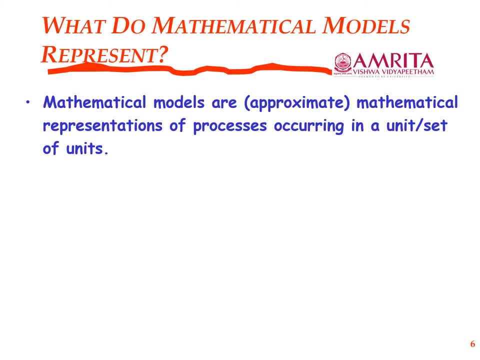 established. in the thermal sense the temperature is essentially equal. that is a very good approximation. mechanically also, it is a very good approximation that the vapor and the liquid phases are in almost the same pressure. chemically equilibrium, not a whole lot, i mean. yes, there would be some stage efficiency you want to maximize. 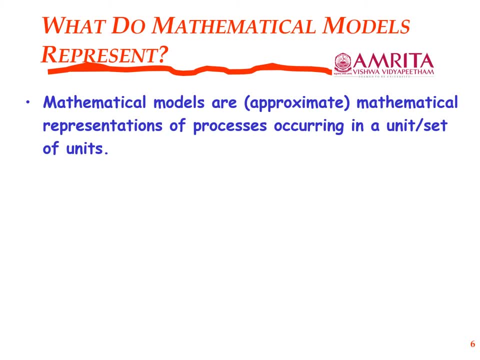 that stage, efficiency as much as possible. and so, in all of these manners, you know we are writing equilibrium relations. they are, they are not necessarily fully met in the unit and therefore those are approximations and, um, you know, therefore, we, when we write that there is the total masses conserved, the species, 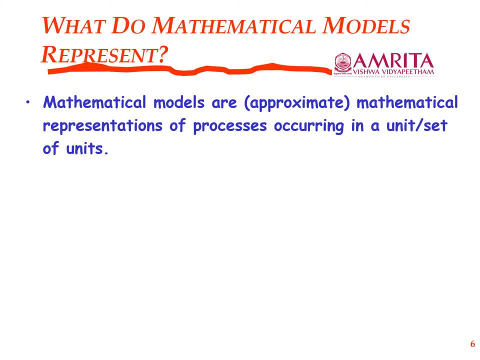 are conserved and the energy is conserved. yes, they are conserved. conservation is exact, but we partition the total energy into those assigned to different streams. we say that the vapor has a vapor stream leaving the tray has a certain enthalpy. the liquid stream leaving the tray 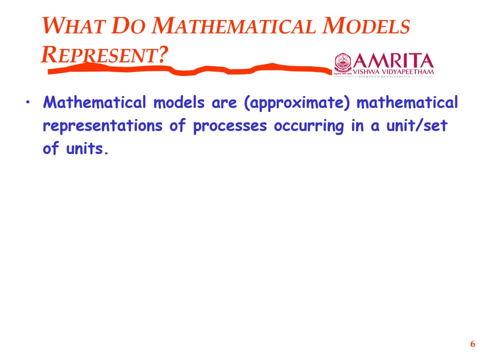 has a certain enthalpy. the vapor stream entering the spray has a certain enthalpy. the liquid stream entering the tray has a certain enthalpy. this distribution of the total energy, that is of the content that is present in the system, that distribution is approximate, because we do not exactly know. 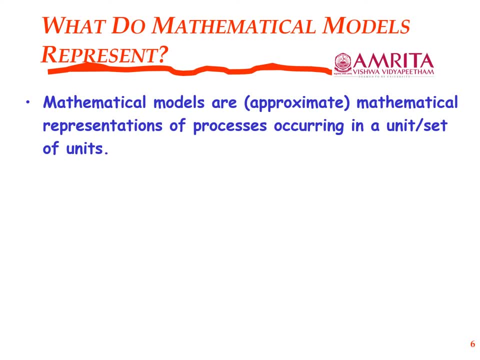 the local variations in temperatures, local variations in pressures, local variations in compositions, and therefore there is approximations that come in even into those conservation equations in the way we assign numbers to them. ok, So, yes, there are, there is approximation, mathematical representation, yes, all kinds of equations. 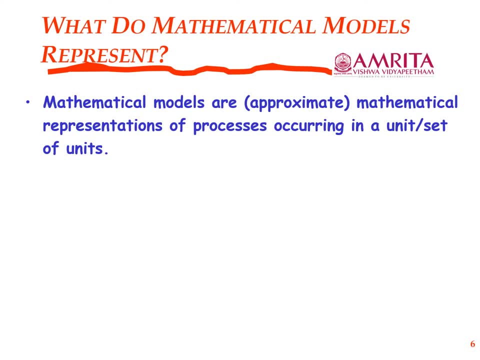 that we, that we saw there right, and then that is. the mathematical model- is an approximate mathematical representation of a set of processes that occur in a unit or a set of units. We can look at various examples. you have studied so many units and processes in your chemical 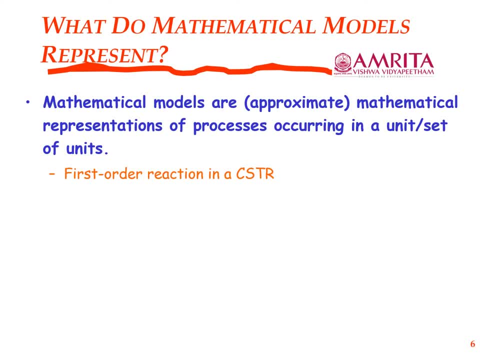 engineering courses so far, and all of them you have described mathematically. This basically means that that mathematical explanation is not only a mathematical representation, but it is also a mathematical representation of a set of processes that occur in a unit or a set of units. 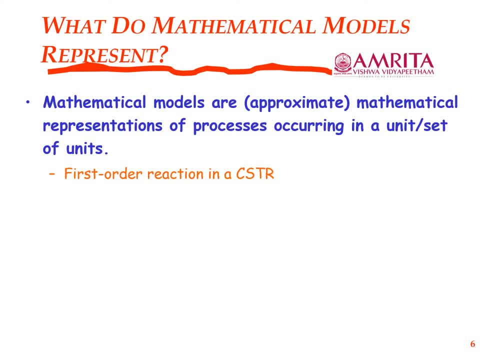 So the mathematical expression is also an approximation. for example, you consider first order reaction in the CSTR that the reaction is first order, that the kinetics is first order is an approximation. that the tank is perfectly mixed flow, an ideal CSTR. or even if you say there is non-ideality, the extent of non-ideality that you are able to capture. 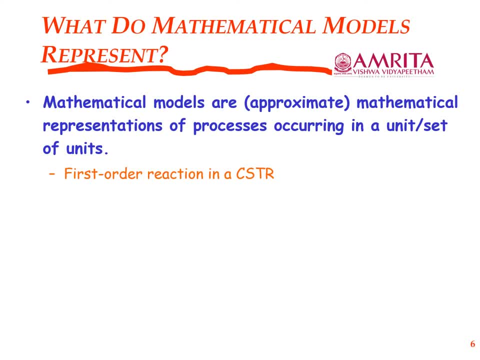 is an approximation, So approximate mathematical representations of a processes occurring in a unit, A distillation of a multi component mixture in a tributary. Here in a tray tower column of equilibrium stages are traced. we just discussed this: Heat transfer in a shell and tube heat exchanger in a countercurrent flow. well, again, the countercurrent. 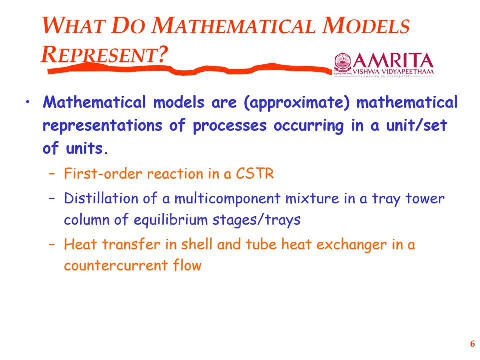 idea is an approximation and you assume that the flow is plug flow because you usually have a velocity, constant velocity, that you assign to the hot stream and the cold stream. that is an approximation and the heat transfer coefficient is an approximate measurement right And therefore the correlations, the correlations between the hot stream and the cold stream. 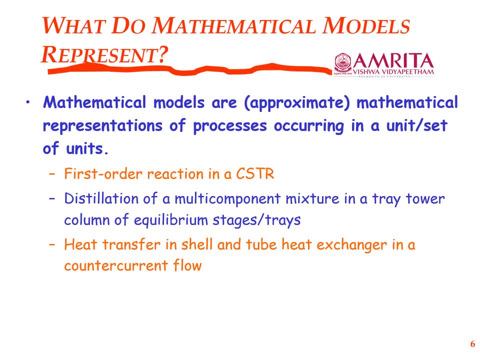 that is an approximation, and the heat transfer coefficient is an approximate measurement, right? So you have the correlations that you use for your massite number and Reynolds number, Prandtl number, which with which you sort of design these exchanges approximations, the geometry approximation, and so on, so forth. 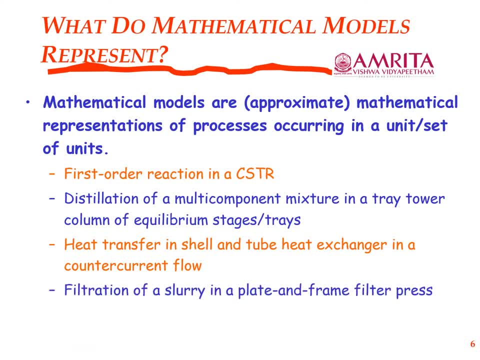 But you capture all that behavior using some mathematical representations: Filtration of a slurry in a plate and frame filter press. one of the most common approximations that you will make is that the filter cake has a certain uniform porosity, which of course is not true, right? 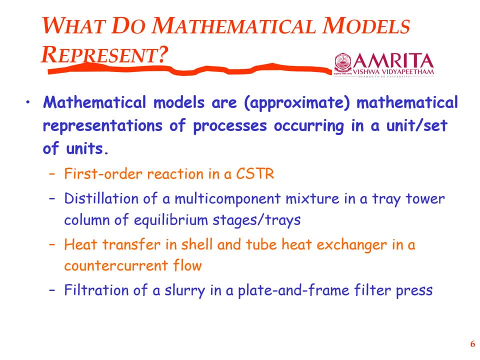 And the slurry, The slurry, The slurry that is coming in has a uniform dispersion of the solid particles, which of course is not true, right. But within those approximations you write mathematical representations, you write something like a Darcy's law, and so on, so forth. 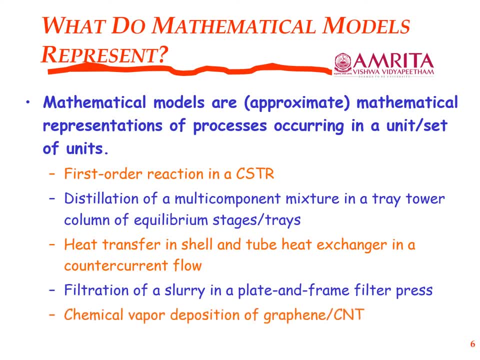 So there you are again approximate representation of some real process. Chemical vapor deposition of a graphene or carbon nanotubes is something that we will discuss, whether we discuss it for graphene or for some other processes like semiconductor fab, like silicon deposition or something like that. 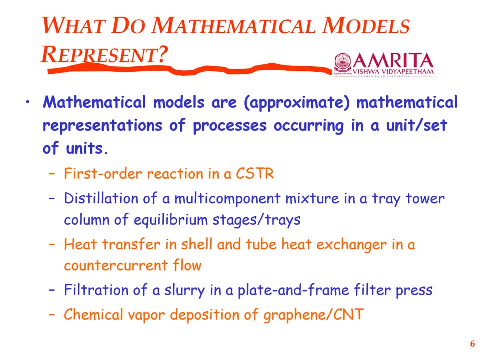 All right, we can. we take up one CVD example as a model. at some point I will discuss this in more detail. I just wanted to put an example of something that is more sophisticated, recent sort of process development: Spreading of a virus during a pandemic. I mean you know this, this whole thing, this whole. 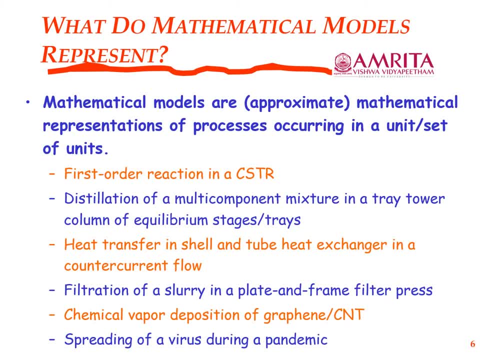 lectures are being recorded at the time that we are all going through a corona covid 19 virus pandemic. And how does this work? How does this work? So there is a virus spread and there are all kinds of predictions that are going around, which are all based on mathematical models, and there are lots of approximations that 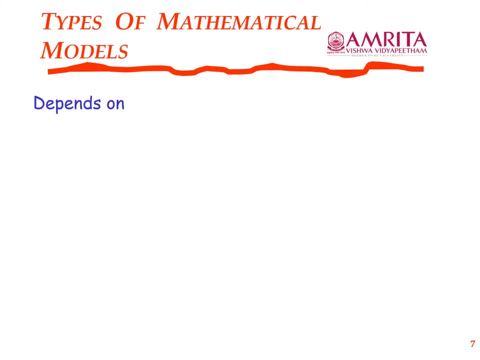 go into those models. So the types of mathematical model depends on the nature of the process. So, depending on the nature of the process, you can characterize some model to be either a deterministic model or a stochastic model. A stochastic model is a model that allows for fluctuations in variables. 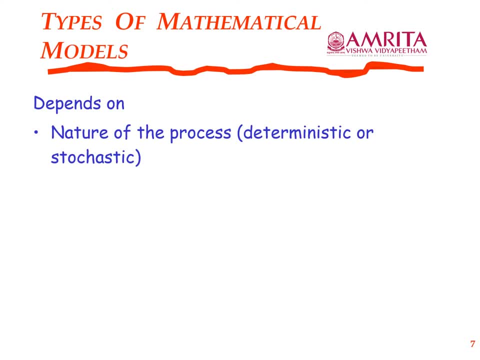 It allows for fluctuations in variables Or random fluctuations in variables, and therefore the model involves random variables, whereas deterministic models involve absolutely determinable certain variables with no scope for fluctuations. It is basically the kind of assumption that you make. so you know you look at a process. 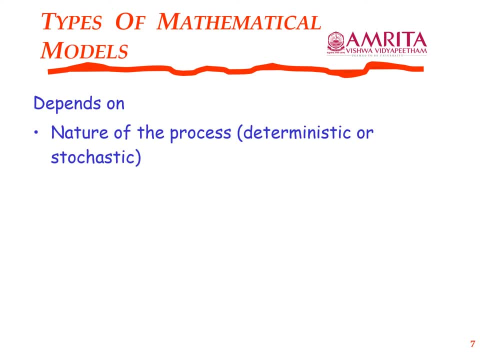 The same CSPR. if you look at it as an ideal CSPR, the model that you develop is a deterministic model. So when you start talking about residence time distribution and there is a non-ideality in the CSPR and you want to capture it, the whole model becomes a stochastic model. 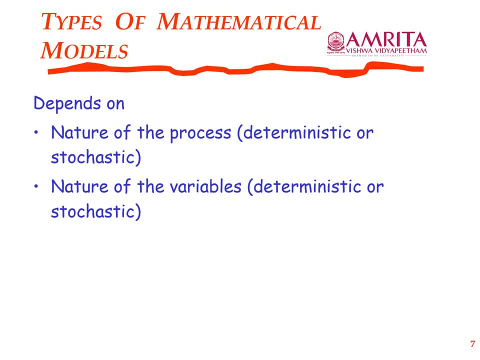 Nature of the variables also- and, yes, this, of course, the example that I gave you now is with the CSPR- is one of- is one of a certain process that is deterministic or stochastic, in the sense that the path, The path Is traced by the fluid particles in a CSPR right when they, from the time they enter to 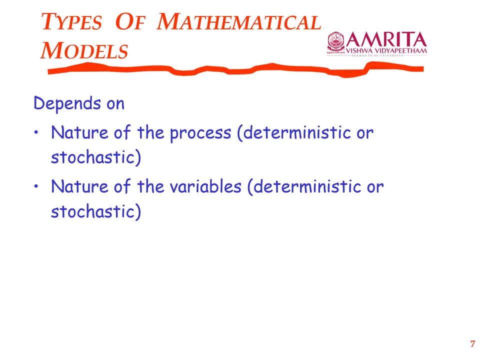 the time they leave that path trace. the flow process is a stochastic process and therefore that is captured by a stochastic variable which you define to be the residence time of that particular fluid particle. and then you look at the residence time distribution of all the particles that you collect at the exit. 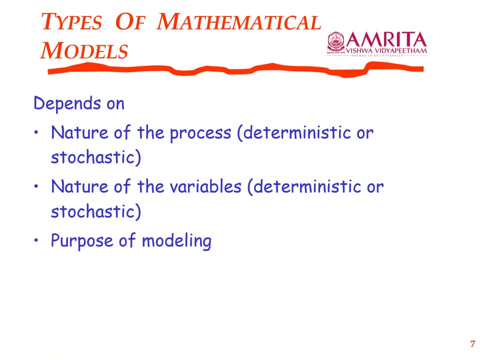 So nature of the process, Of the variable and depending on the purpose of the model. so you can either have a descriptive model or a prescriptive model, and the descriptive model is one of process identification. you will try and take up one example of process identification model at some point in this. 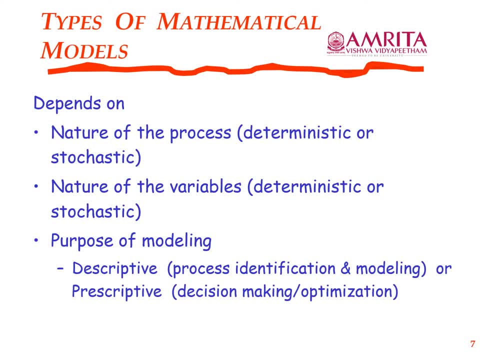 course, but a prescriptive model is what we typically usually come up with, where you can predict prescriptive models, can they have some sort of a predictive power and therefore you can use those models To make decisions, use those models to optimize. on the other hand, descriptive model is a model. 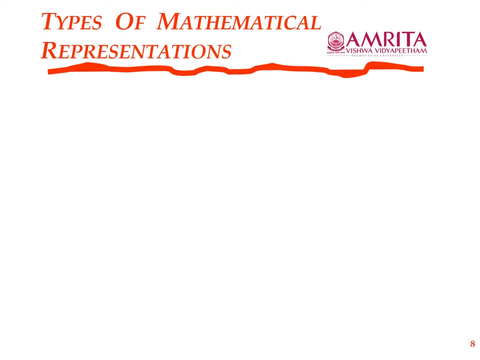 that is that is developed to identify the nature of the path. What are the different types of mathematical representations? yeah, you can write equations, which is what we saw. sometimes you can have inequalities. this is something that we saw in the first lecture, when we were looking at some sort of constraints on what can be. 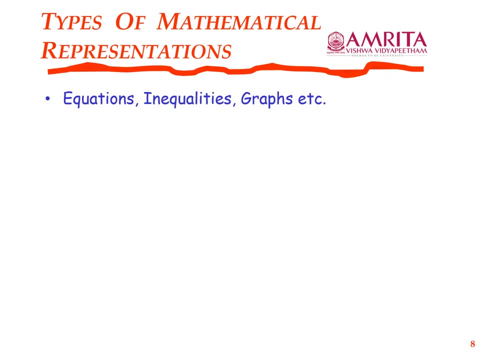 the outlet temperature or inlet temperature to react Inlet composition of an inert species into a reactor, especially when the reactor has recycled, and so on so forth. This temperature cannot be greater than 150 degrees or your inert composition cannot exceed one mole percent or two mole percent or whatever it is. 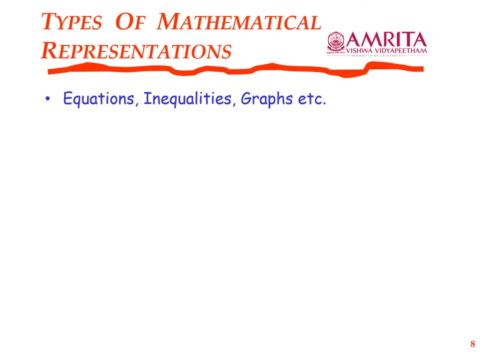 So those are all in inequalities, and then you can also represent, you know multi, you know sort of a large process of multiple units as graphs. And this graphs- I am not talking about the- the graph that describes, you know a graphical way of describing, what is the relationship between one variable and then another variable. 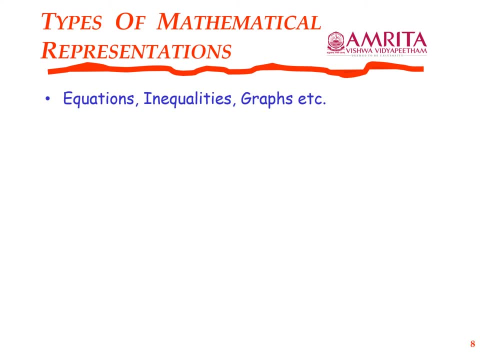 that is also a graph, but I am also talking. I am talking about these various nodes and edges that connect each other and then they form a certain certain shape, right. So those kind of graphs can also be used in mathematical representations. If you are looking at equations, you can have either linear algebraic equations or non-linear. 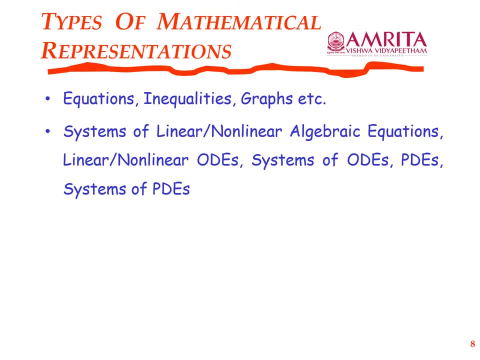 equations: Non-linear algebraic equations, single equation or the system of equation. linear ordinary differential equation, non-linear ordinary differential equations are systems of such ordinary differential equations, systems of partial differential equations, inequality constraints, as I was saying in optimization problems, and systems of a mixture of these. 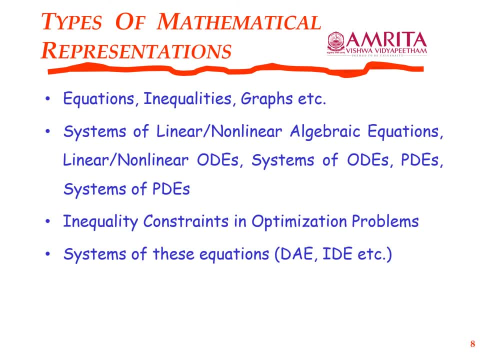 equations, basically some algebraic equation and some ordinary differential equation, non-linear algebraic equation, non-linear partial differential equations. So these are all basically differential algebraic equations, that is, VAE or integro differential equations. you can even have integral equations. all right, When you have your RTD, your concentration, exit concentration is given by a convolution. 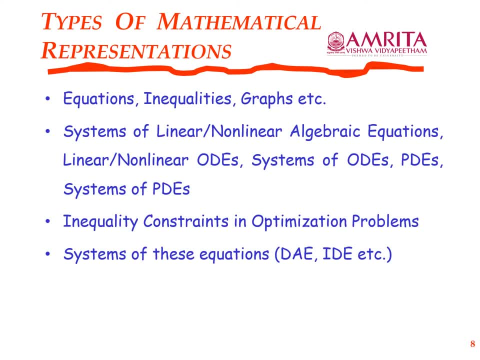 integral right of the E distribution which is your at residence time distribution, that is, you know, multiply that with that is the probability distribution, and then multiply it with your concentration of the that particular fluid particle of the inlet, and then you integrate over various times from the inlet to outlet. 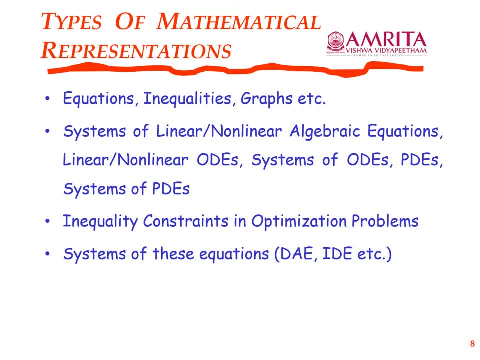 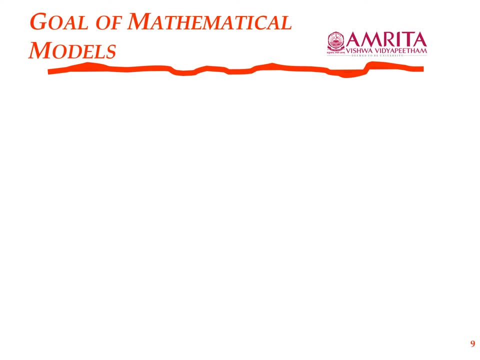 So you get basically an integral equation for the exit concentration. You can have some equations that are differential equations and some equations that are integral equations, and therefore you can have integro differential equations. But given all of these equations, what is the goal of a VE? 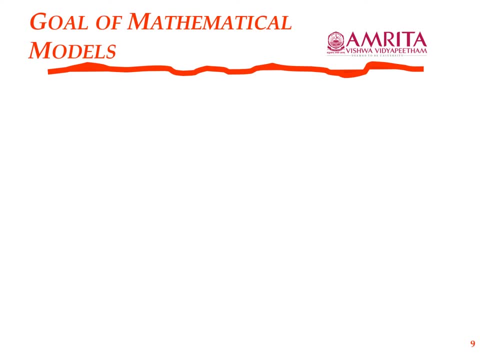 What is the ultimate purpose of writing mathematical models? So the purpose of mathematical model is to establish a relationship between the inputs to the system and the outputs from the system. right? this could be singular or plural, doesn't matter. inputs, outputs, right? So you want to be able to express some form of a relationship, either a direct relationship, 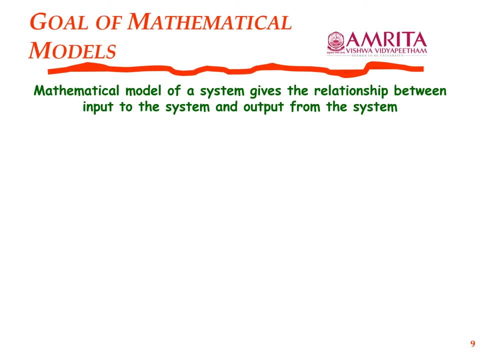 or an indirect relationship. either you write: you know y is equal to Ax plus b, that is a direct relationship between y and x. and indirect relationship is to say that dy by dx equal to ax plus bx square. So you know, you can. you have to integrate that equation to get the direct relationship. 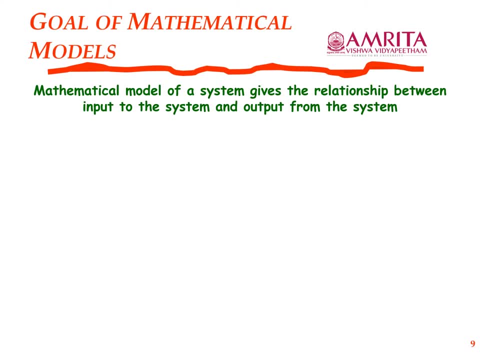 that is so. therefore, basically, you know you want to establish some form of a relationship between the inputs to the system and the outputs from the system, and so here I want to talk about a central idea In developing mathematically models. ok, So here is. here is the mathematical model of a unit or a process. there is a box at the 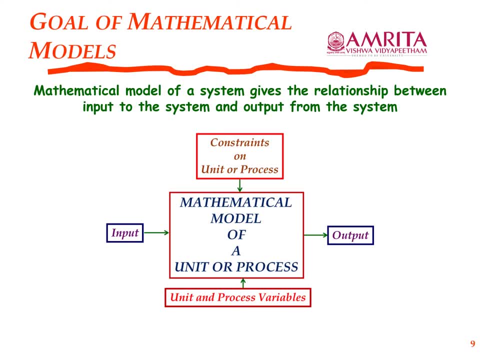 center and I this. this picture we will see repeatedly. all right, there are some inputs that go into the model, there are some outputs that come from the model and then there are. so you are, you are, you are. you have some variables that describe the process that takes place. 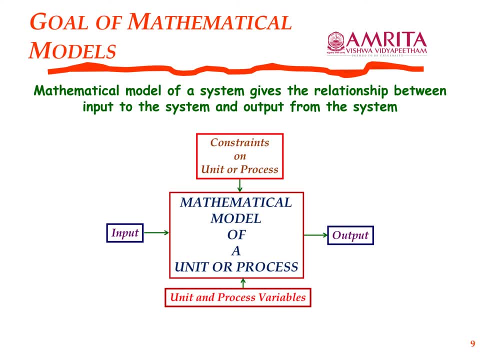 in a unit which you are trying to model. So let us let me rephrase this: The mathematical model is an approximate mathematical representation of the various processes that occur in a single unit or a set of units. right, So there are variables that describe the process. For example, you are talking about a chemical. 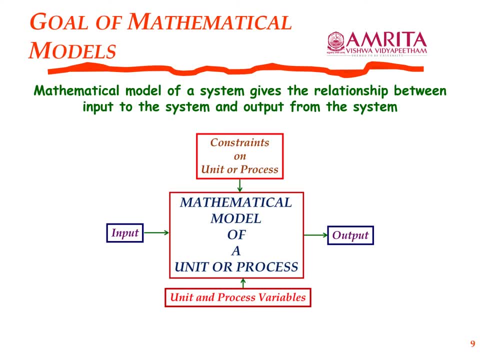 reaction. at what temperature is this reaction taking place? at what pressure is this reaction taking place? what is the rate constant for this chemical reaction? what is the order of this chemical reaction? these are all process variables. And what about the unit variables? where is this reaction taking place? in a CSTR, So? 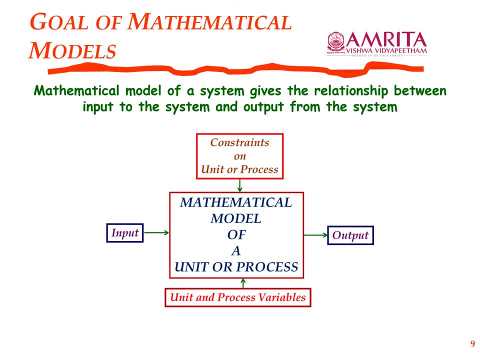 what is the volume of the CSTR, If it is PFR, what is the cross sectional area and what is the length? and what are the input variables? what is the inlet concentration, what is the temperature, what is the pressure of the input stream? and what about the outputs? 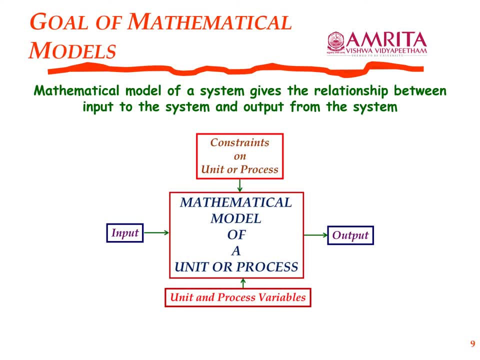 variable, what are? what is the outlet concentration, which means of course you can calculate what is the output conversion right from that CSTR or PFR, and what unit, all right. and what is the temperature, what is the pressure, what is the flow rate of the output stream, and then the mathematical model itself becomes some form of a relationship between all. 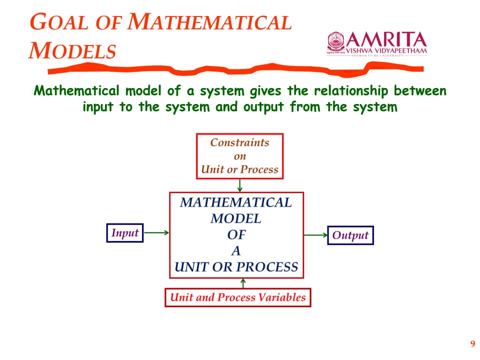 these variables and they are explained, expressed as constraints on the unit or the process. so, okay, so you, you, you basically specify, for example, in one way of solving a csdr problem. you would have done this, you know. you specify the volume of the reactor and you ask what is? 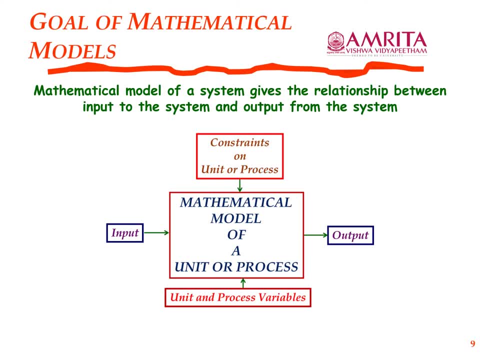 the output concentration or what is the conversion from the csdr. so basically you can specify the constraint on a unit and constraint on a process. you say that the rate constant is given by this value, okay, or some expression which is a function of temperature, and you know you have your input. 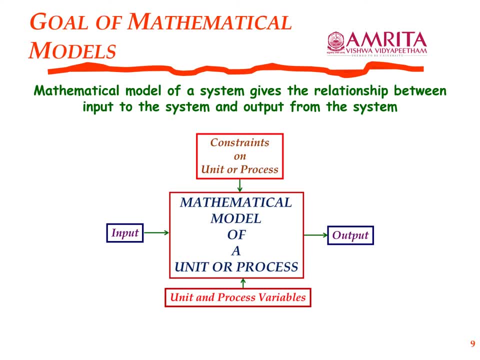 stream, and then you have your unit process variables that have given volume is given, temperature is given, at least the reaction take place is given, and then calculate the conversion. or you can have, for example, your conversion is given, tell me what should be the volume of the csdr to achieve. 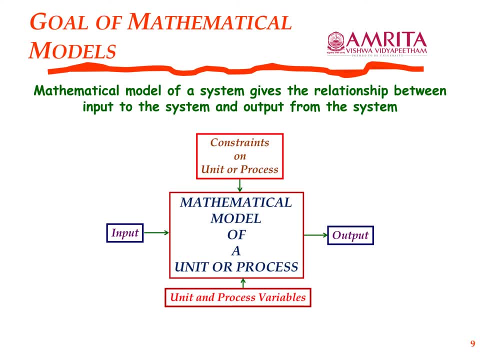 that conversion. you have done all these kinds of problems so ultimately, to solve such problems, you need to have these constraints or these equations. it could be equations, they could be inequalities, equality or inequality, constraints, different types of equations that we just saw in a couple of slides ago. right so? 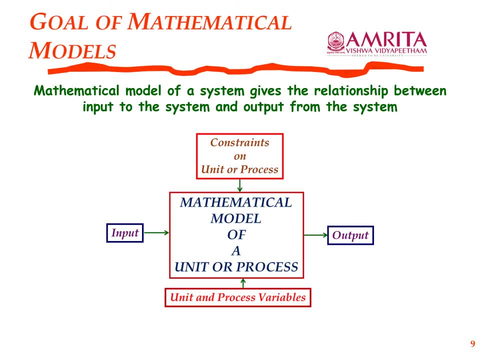 this basic framework is how you can envision any mathematical model. so the moment you are asked to model any system, you should first ask yourself: what are all the input, inputs that go into the unit or a process? all right, or rather i should, i should back up and say this: 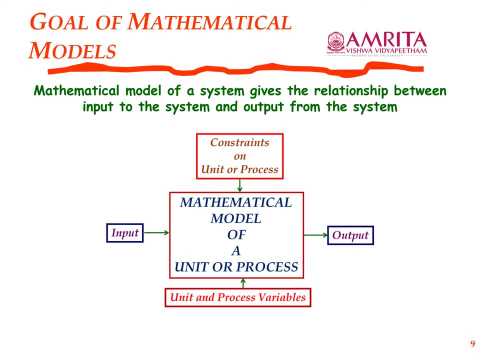 the moment you are asked to develop a mathematical model for some process or processes that are taking place in one unit or a system units, you have to ask yourself what are all the that go into that unit? are the systems of units? and you should ask yourself what are all the outputs that come out of that unit? are the system of units? 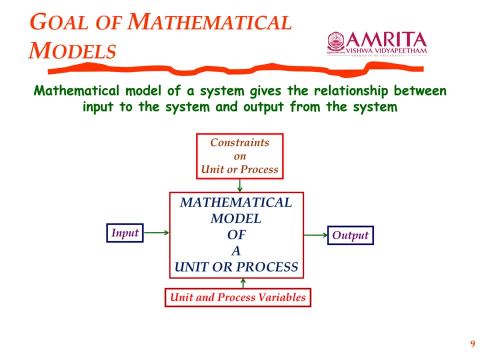 and you have to then ask yourselves: what are all the variables that I can use to describe that unit or system of units, and what are all the variables I can write I can use to describe the processes that take place in that unit or system of units? once you've defined all these variables, then you start. 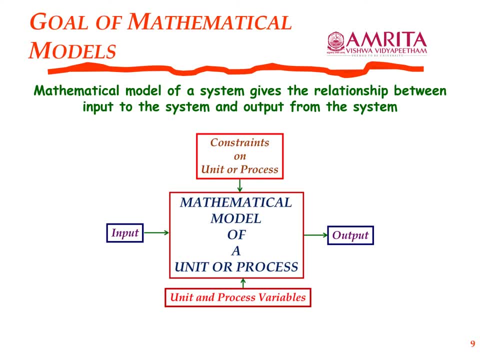 looking at what sort of constraints, equations or inequalities that relate these variables, and then you simplify that, you get a mathematical model which you simulate or solve, all right. so this sort of a systematic approach we will take in this course and the the. the core idea is therefore that whole systematic approach is therefore distilled. 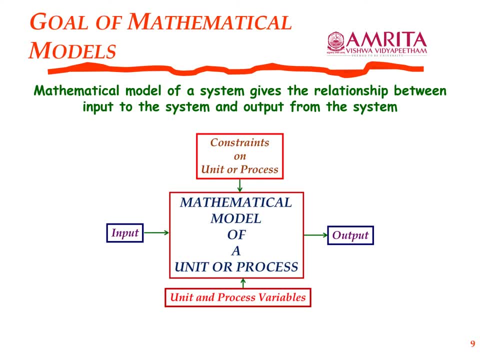 in this block diagram that describes how mathematical modeling works. so here is what you aim at. you know, ideally you would like to see output as a function of this various input stream variables, the unit variables and process variables. sometimes you will be asked to calculate the unit variables given a certain output. so you know you, you may have to, in, you know, invert this function. 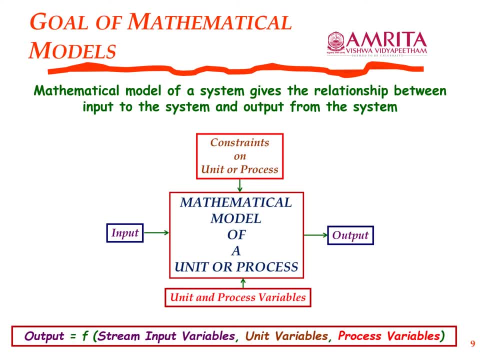 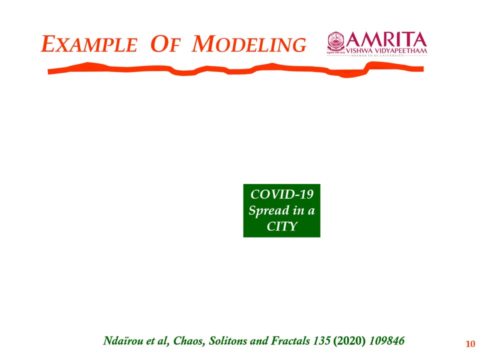 in some form or the other, but this is what happens. you know, this is the sort of goal of a mathematical model to express a relationship like this. now, to close picture, i am going to give one example of modeling, and that is pertinent to what is happening right now. 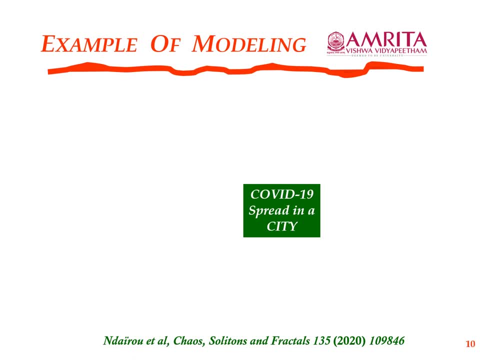 where we are facing a pandemic of corona covid 19 virus. how does this virus spread in a city? and i want to understand this. there has been a recent study whose reference is given to you in this, in the reference below, and uh, based on that- uh, you know- study. i'm not going to show any equations here, but i'm going. 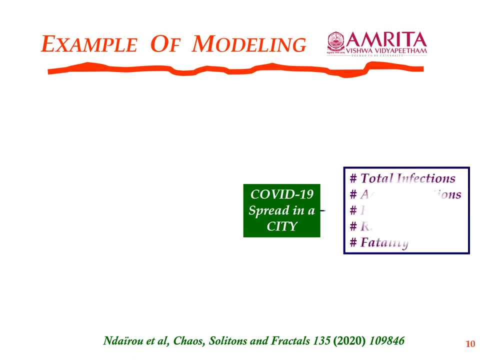 to show the block diagram, so to speak. so, basically, what are the outputs that you are looking at? what is the total number of infections? what is the number of active infections? how many of these active infections are hospitalized, how many of the total infections have recovered and how many of the total infection in infectious patients have? unfortunately, 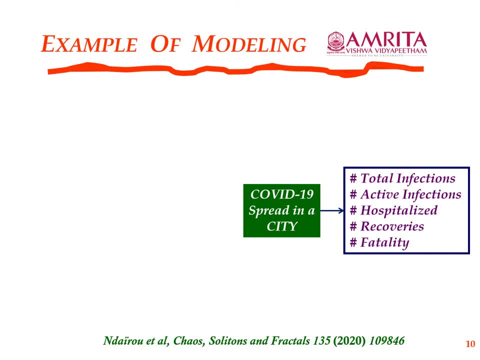 passed away. so these are the kind of information that you want to learn and track. all right, this is what the model should be able to predict. these are the outputs. what is the input? who are all the susceptible people? who are all the exposed people out of these exposed people? 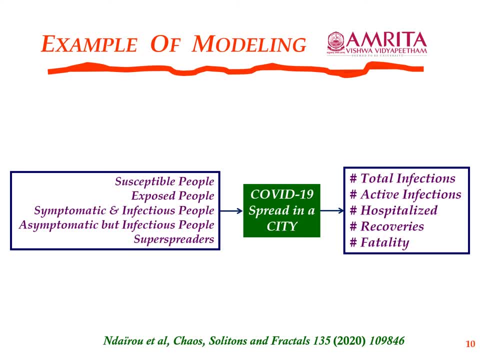 how many have become infectious and are exhibiting symptoms of covid 19? how many have become infected, infectious but are not asymptomatic? and then, as we have seen, there are these class of people: by simply by their virtue of their profession or their travel, history and whatnot, all right they become in, you know. 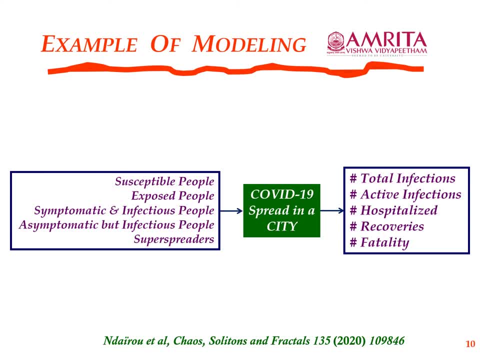 inadvertently exposed, they become super spreaders, right, you know they. you know there was this example of how an outbreak happened in in a large market and then people just picked up you know goods wholesale and they went and sold at different places and they transmitted the virus completely unintentionally. but 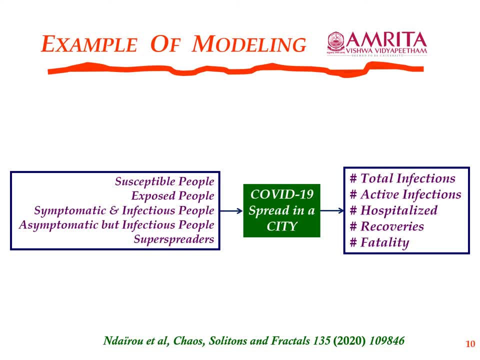 they did end up becoming super spreaders. so one person ended up exposing a whole lot of people compared to what would have happened if that person's profession they are not that particular profession. so we have to account for such such- you know cases of super spreaders also. so these are all the. 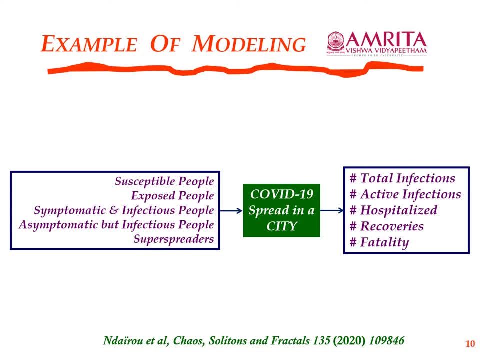 inputs and using this inputs you want to predict this outputs, and for that you have to understand some sort of- you know- unit variable and process variables. what are the unit variables in a given city? what is the population demographics you know? you also have to know the population density. where the population density 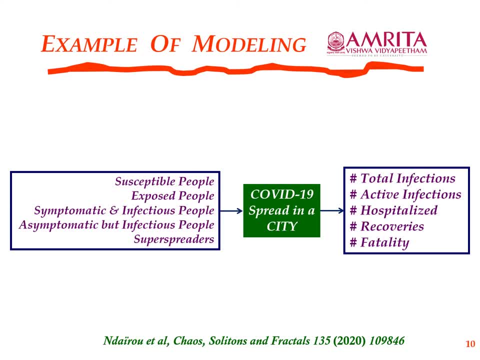 distribution, which areas are sparsely populated, which areas are densely populated, and so on, so forth. and how is the city planning? you know what is the way in which these population is going to come and interact with each other. what is the health care infrastructure, what is the administrative? 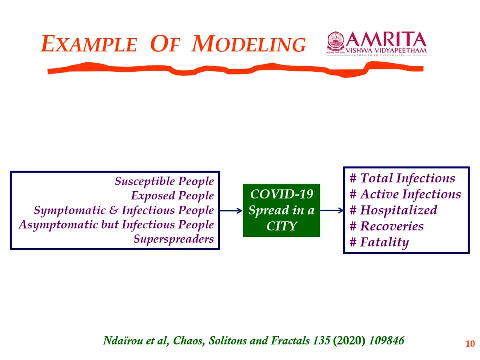 infrastructure? what is the police security infrastructure? what are the jobs and employment infrastructure? what kind of jobs are available? see, I was just talking about the supermarket, you know. so if this, this place, is like one major place where a large number of such, you know, agricultural produce or other, 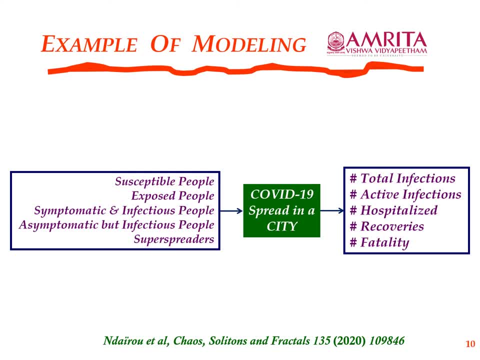 produce sold, and then it's a manufacturing hub or whatever it is. so there will be these kind of concentrations through which such super spreading could happen. right, and what are the shopping infrastructure and how? how much of the shopping infrastructure is working, how it is working? all of this is going to. 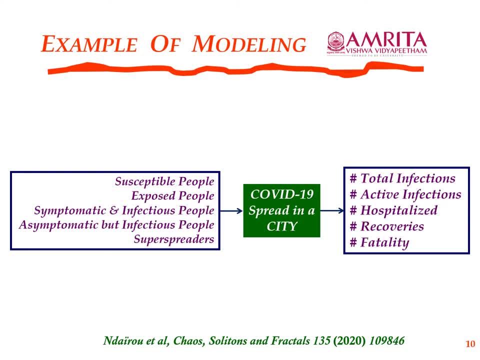 determine how susceptible people who get exposed become infectious, symptomatic or asymptomatic, and then how super spreaders could emerge, and in turn, this, will you know, determine at any point in time in the city the total number of infections, the number of active infections and so on. so forth, right and 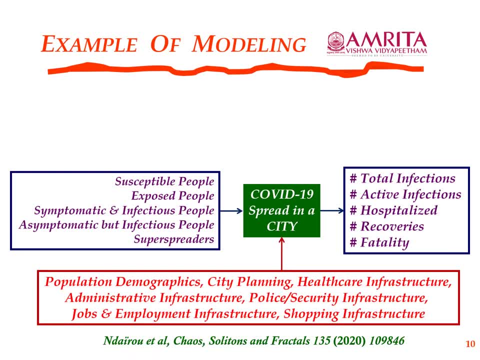 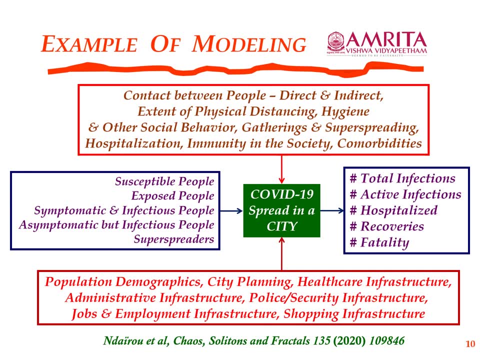 so what are all the constraints? what are all the constraints that we are looking at? the constraints that we are looking at is okay. so what kind of contact exists between people? direct contact or indirect contact? what is the extent of physical distancing that is being observed in the community? what kind of 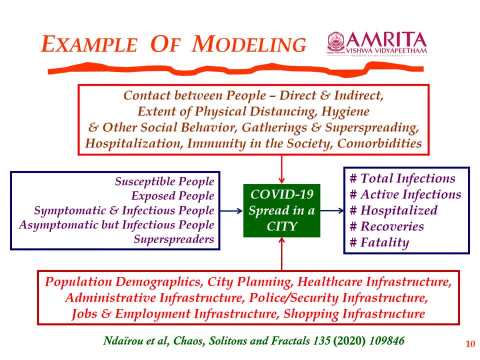 hygiene and social behavior is observed in the community? what kind of gatherings take place and what are the potential for super spreading? what kind of hospitalization is taking place? are the infectious people, if at all, especially when they are symptomatic? are they getting hospitalized? what is the general immunity in this cycle and that? 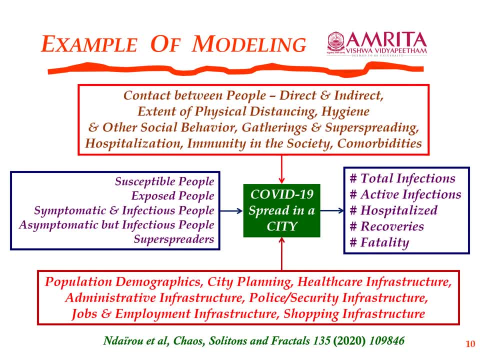 that plays a major role, that receives a big difference worldwide. if you look at some, some countries seem to be surprisingly more capable of resisting this virus. why, if something may be discovered much, much later- but that is a reality to me that we are facing- and what are the comorbidities for the 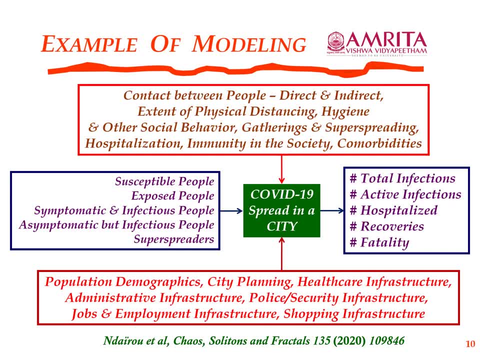 people, who who are susceptible, who are exposed, who are infectious, that could cause the people to become symptomatic and for those symptomatic people to become very serious, to the point that recovery may not be possible and fatalities may occur. so all of these are constraints, so we have to have ways to express each of this, mathematically speaking, right and then find a way. 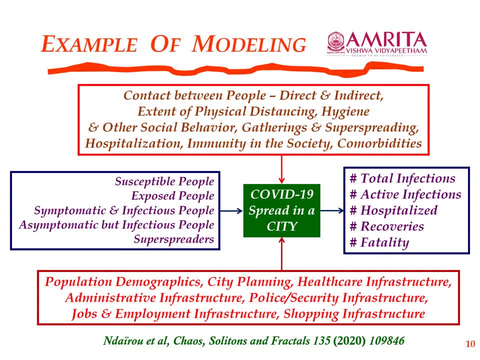 to develop a set of equations that relate the output. i want to know total infections as a function of all these three the: the ones in the purple uh font on the left side, the brown font the top, the red fonts at the bottom, all of these, how does the number of recoveries depend on the 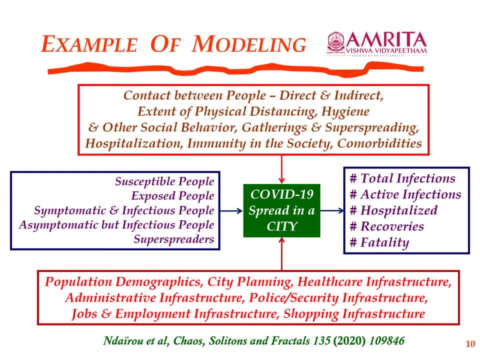 number of susceptible people, number of exposed people, number of symptomatic infectious people and so on, so forth. how does the number of recoveries depend on population demographics, job and employment infrastructure, police security infrastructure, obviously healthcare infrastructure? how does the number of recovery depend on the percentage hospitalization, the nature of immunities, the 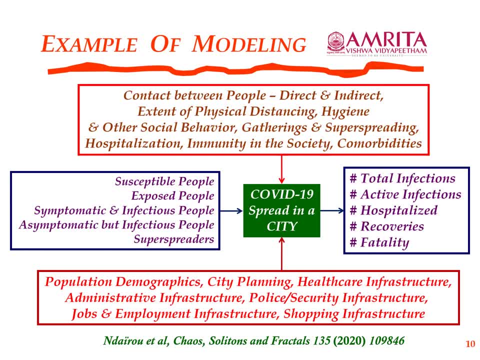 nature of comorbidities and so on, so forth. so there has to be some sort of equations that will have to be developed for all of these. that would be the model, mathematical model, for predicting. this would be the model for predicting the number of recovered people. 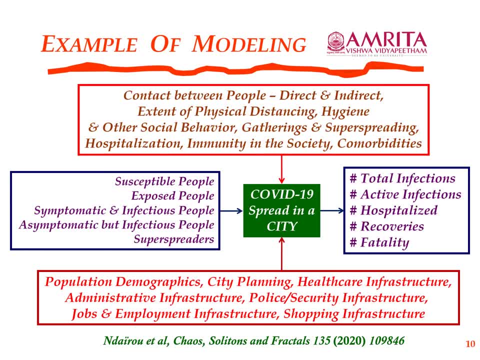 that would be a prescriptive, predictive model that describes the uh, that predicts how the covid19 coronavirus is likely to spread in any given city, and this paper that is cited below is an example, is a very good example of how such a model could be developed. all right, so this- this 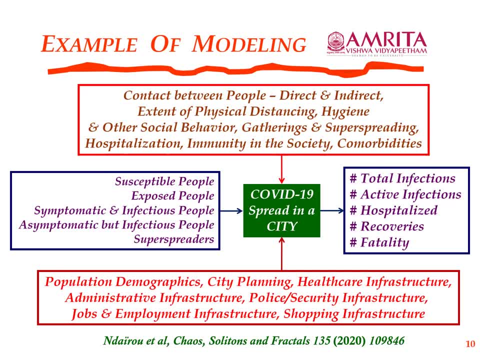 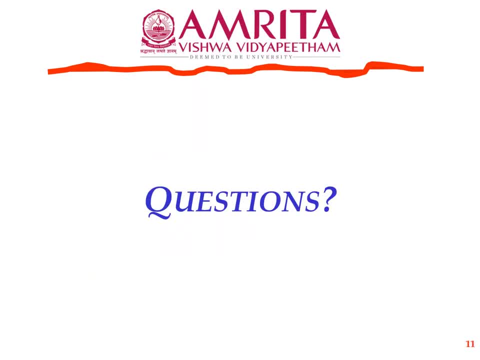 is the kind of mathematical modeling that we are trying to learn, of course, with respect to chemical engineering systems, and we are trying to learn, of course, with respect to chemical engineering systems in this course. so, um, if you have any questions, you can, you may please post those questions in the 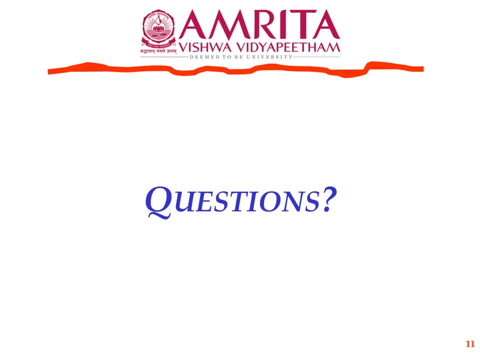 comment section below. and, um, you know, uh, i hope you are able to understand how mathematical models are constructed, what are all the various pieces in the puzzle, how they they work in in achieving certain specific goals, in terms of either describing a system or prescribing predictive models, or predicting how a system will behave and using which you can take decisions you can have. 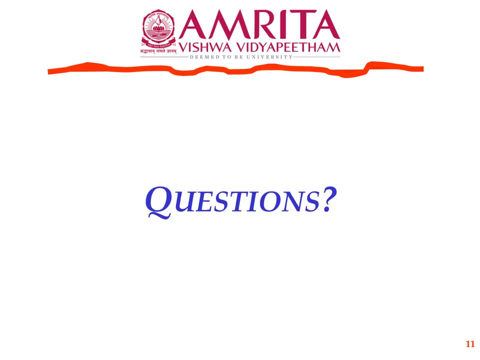 mathematical models that can be used as decisions, the decisions themselves can be expressed mathematically, and so on, so forth. right, so um, with this, i would like to thank you for, you know, listening to this lecture. please give your feedback and, uh, looking forward to interacting with you in the next lecture. thank you very much. you.